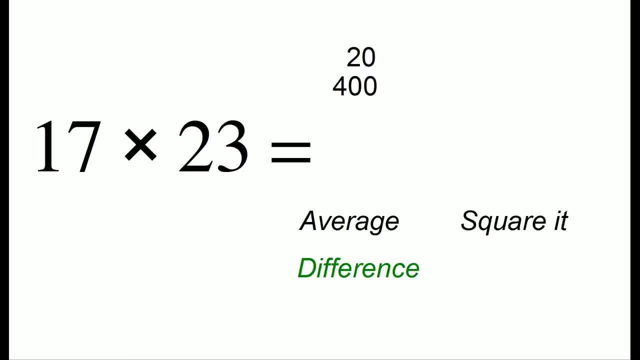 17 and 23 are both 3 away from the average. We then are going to square that difference, and 3 squared is 9.. The final step is we're going to take the square of the average minus the square of the difference. So 400 minus 9 gets us to our answer of 391.. 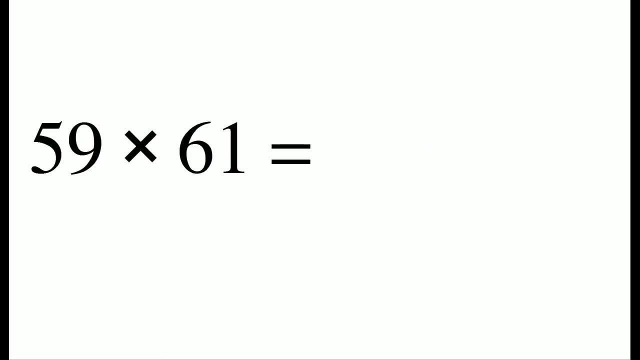 Let's do another example. Let's do 59 times 61. We mentally compute the average of 60. Then we take the square of 3600.. We then look at the difference from the average, which is 1.. We square that, which is also 1.. 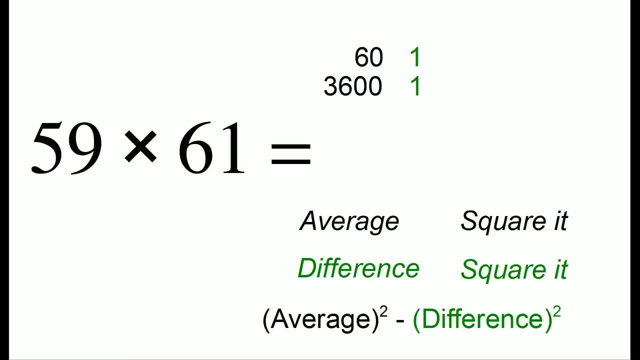 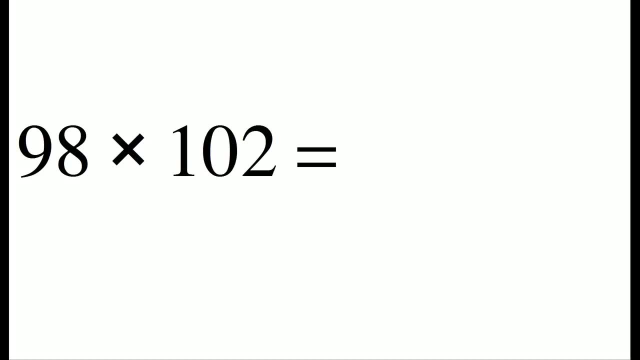 And finally, we take the difference of the squares, which gets us to 3599.. Let's do 98 times 100.. We then look at the difference from the average. We then take the square of 100 and 2.. The average is 100, which we then square, which gets us 10,000.. 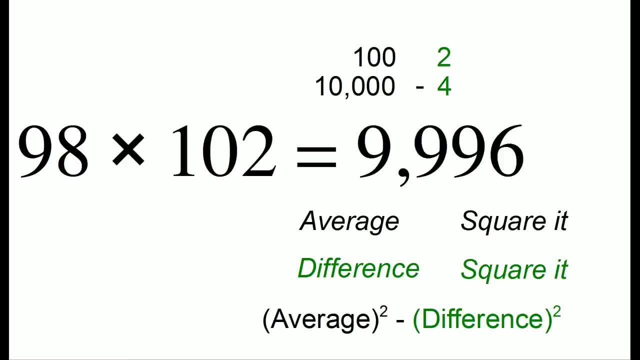 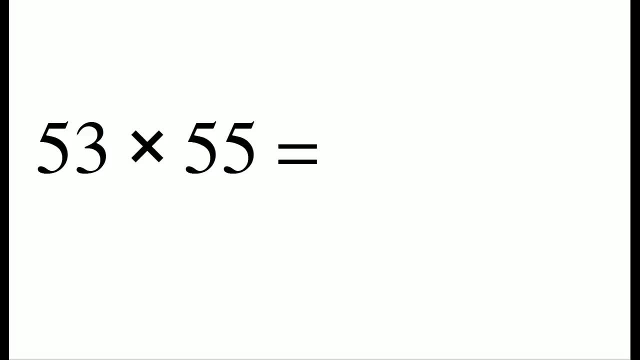 The difference from the average is 2.. Squared is 4. And when we take the difference we get the answer of 9,996.. Let's do another problem. Let's do 53 times 55.. The average is 54.. 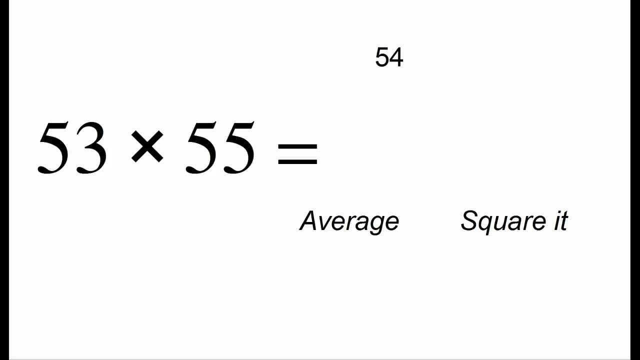 We then look at the difference from the average, which we then need to square. This will be tricky. Most of you don't know how to do this. I actually explained a trick in a previous video of how to square numbers in the 50s. So, combining that trick, we'll go ahead and 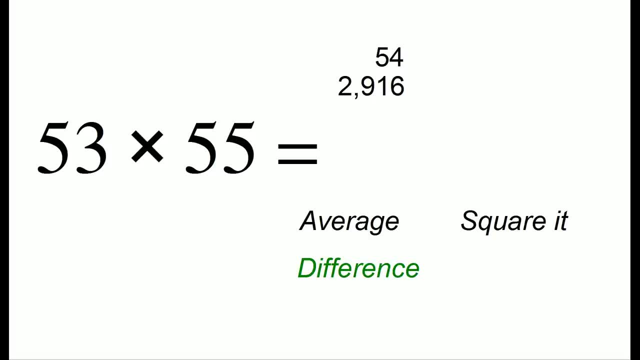 use it. The square of 54 is 2916.. The difference from 54 is 1.. Squared is also 1.. And taking the difference of the squares gives us the answer of 2915.. Why does this trick work? The reason: I'll give you an algebraic proof. When we're taking a number,